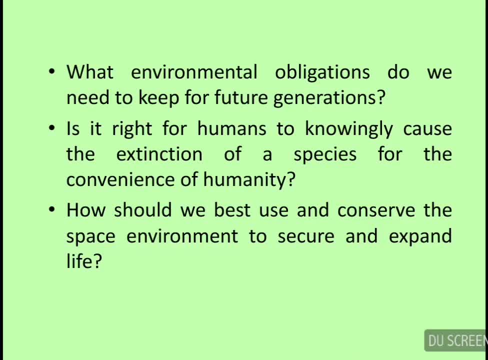 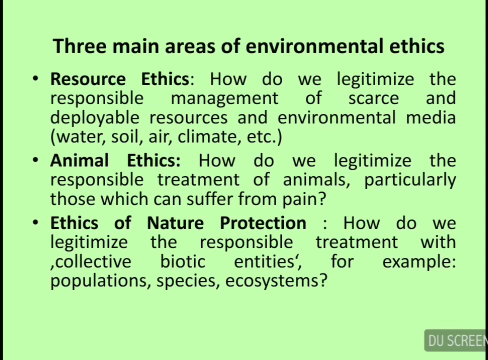 obligations do we need to keep for future generation? Is it right for humans to knowingly cause the extinction of a species for the convenience of humanity? How should we best use and conserve the space environment to secure and expand life? So there are basically three main areas of environmental ethics, that is, resource ethics. 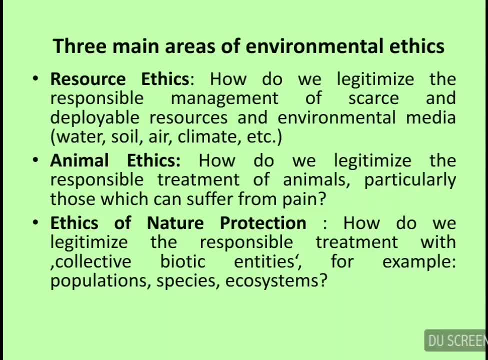 animal ethics and ethics of nature protection. So firstly, we will start with resource ethics: How do we legitimize the responsible management of scarce and deployable resources and environmental media, ie water, soil, air and climate? Animal ethics: How do we legitimize the responsible treatment of animals, particularly those which can suffer? 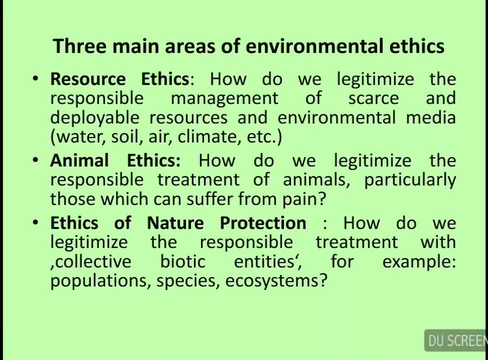 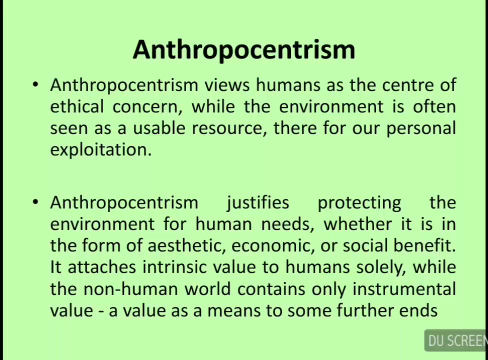 from pain. How do we legitimize the responsible treatment of animals, particularly those which can suffer from pain? We also need to understand the plans of wissenент based conservation: bio22, mic, Technical workers in the tiger & fossil environment, Ethics of Nature Protection. How do we legitimize the responsible treatment? 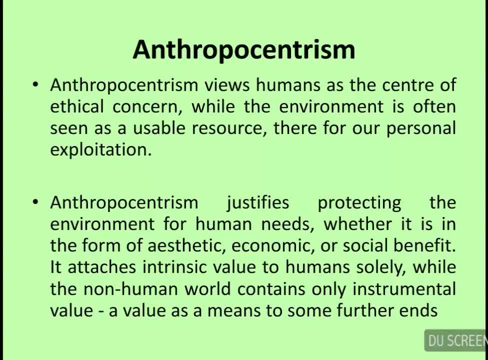 with collective biotech entities, for example population, species and ecosystems. Anthropocentrism: Anthropocentrism views humans as the center of ethical concern, while the environment is often believed to be the üzerine to ethical Ou mind caused concern, behaviour, ideologies, interests, etc. 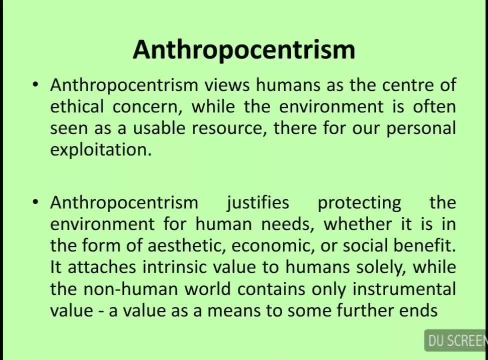 is often seen as a usable resource, Therefore our personal exploitation. Anthropocentrism justifies protecting the environment for the human needs, whether it is in the form of aesthetic, economic or social benefit. It attaches intrinsic value to the humans only, while the non-human word contains only. 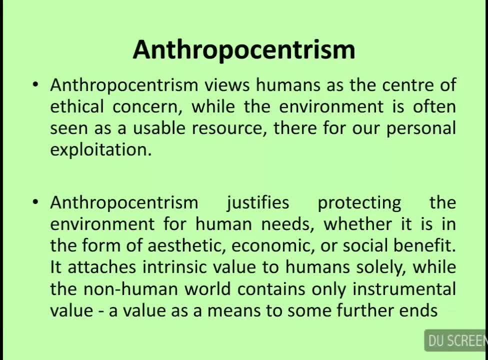 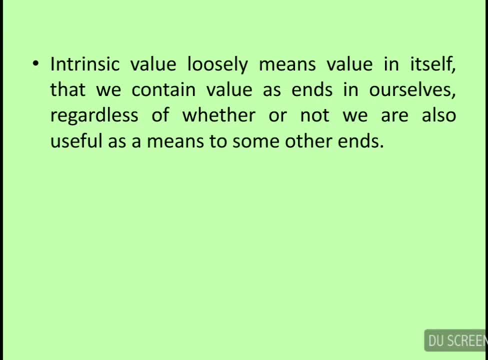 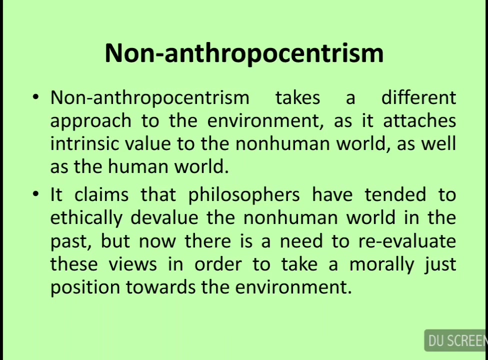 instrumental value of value as a means to some further ends. Intrinsic value loosely means value in itself, That we contain value as ends in ourselves, regardless of whether or not we are also useful as trash means to some other ends. non-anthropocentrism: non-anthropocentrism takes a different approach.